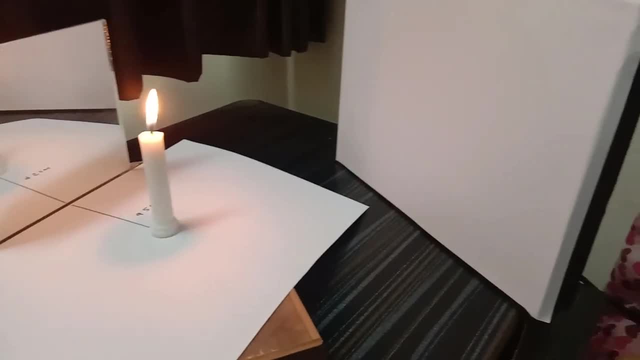 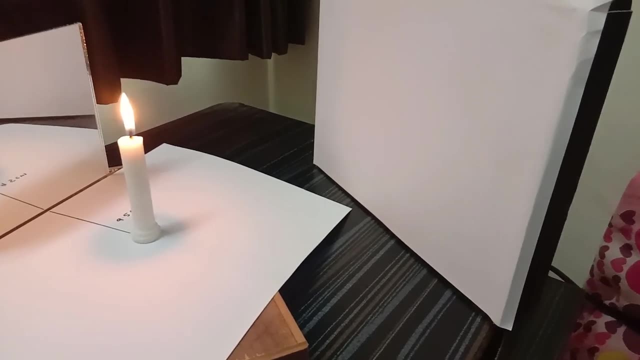 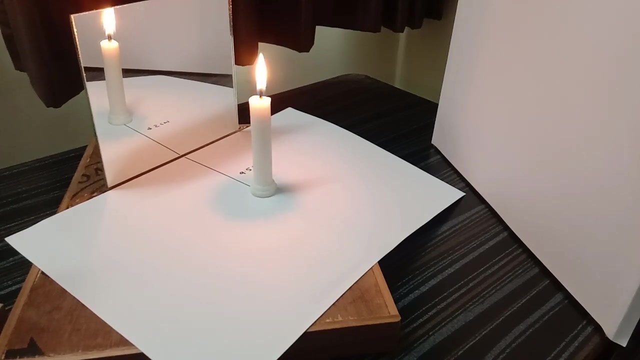 there. Now, here I have taken a white page and I have fixed it on a small box, So that becomes my screen, and I am also going to demonstrate the difference between the virtual image and the real image over here. So, guys, now first of all, let me talk about the properties of the image formed by the 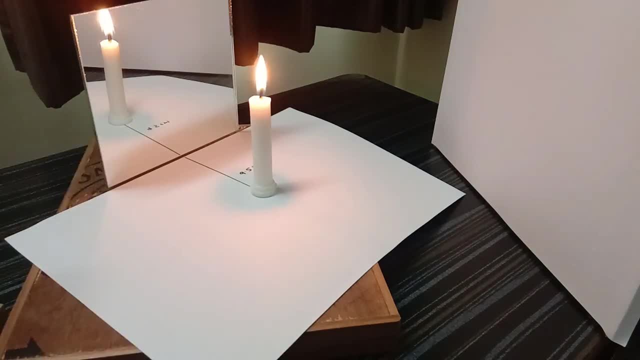 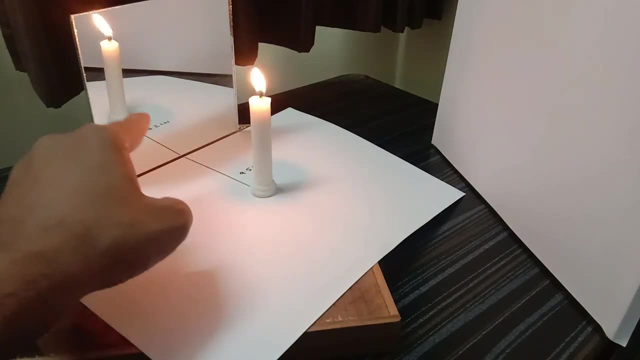 plane mirror. So first is the image is erect. Second thing, the distance from the object to the mirror is same as the distance from the image from the mirror. So if this is at a distance of 9.5 cm, the image is at 9.5 cm behind the mirror. So now let me show. 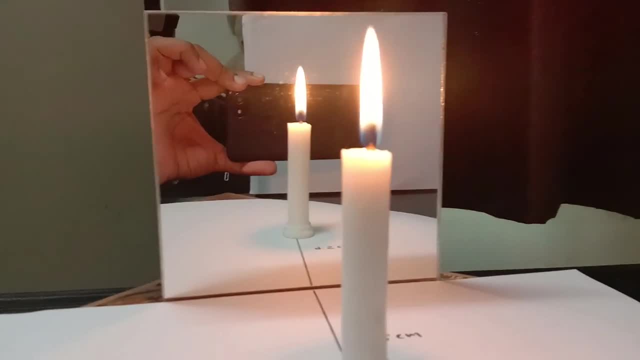 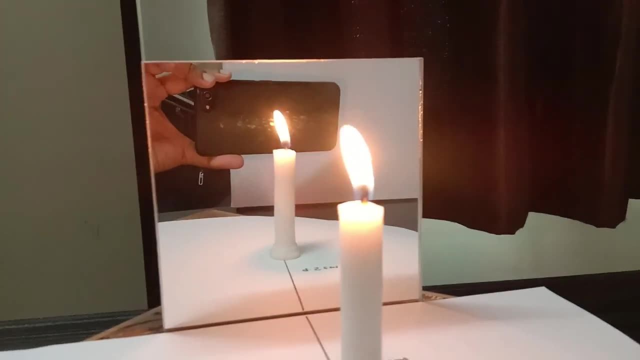 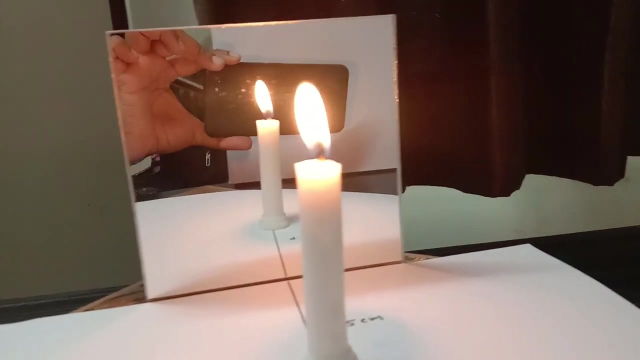 you that It is clearly seen that the height of the object and the height of the image are also the same. You can see that the distance of the object from the mirror and the image from the mirror are same. The another most important point is the height of the image. 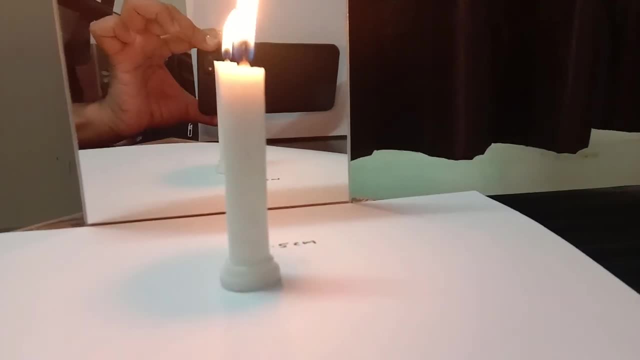 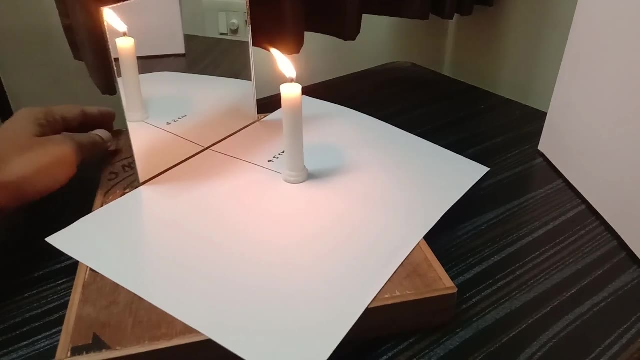 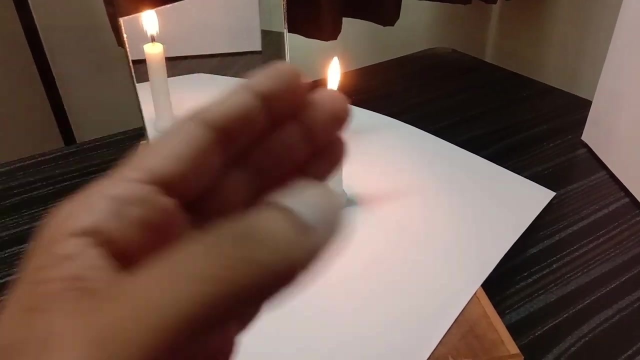 and the height of the object. They are exactly the same. Now, guys, another most important thing to learn from here is we are able to see this image which is behind the mirror. Now, whatever is the background over here behind me, the 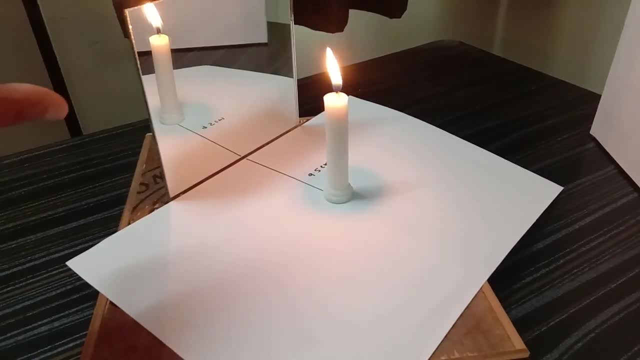 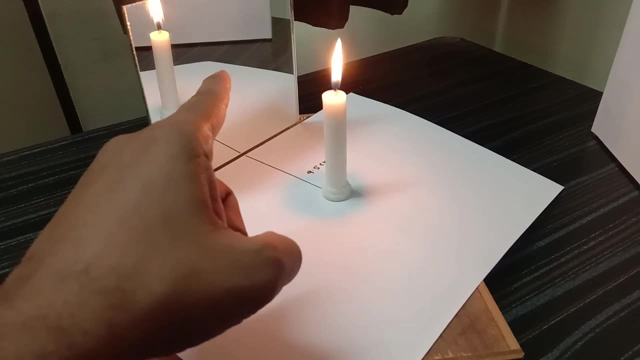 same virtual background appears inside the plane mirror, which is called the virtual world. So this is a fictitious image. This is not a real image. This is the assumption of our mind and this is a virtual image. We are not able to catch it. 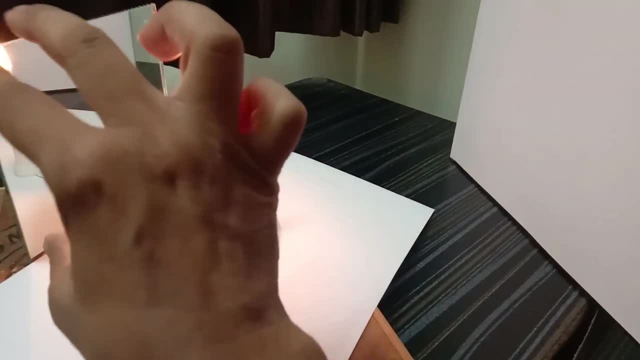 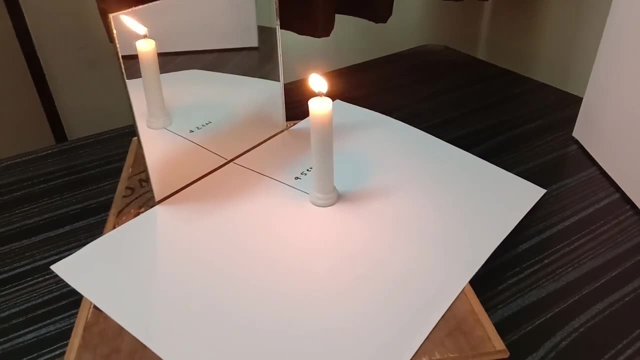 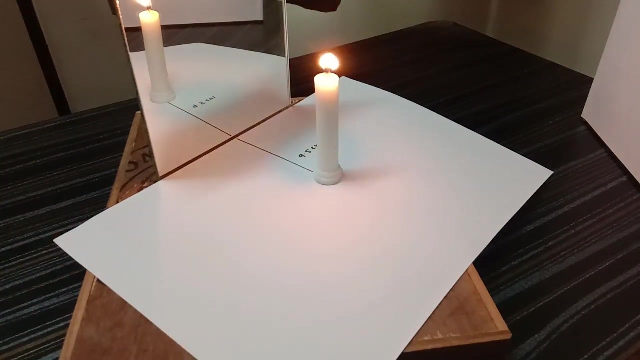 On the screen. you can see that this image which is over there, I am not able to catch it on the screen, So those images which cannot be caught on the screen are referred as the virtual images. guys, Now for a moment, if I remove this plane mirror and if I bring 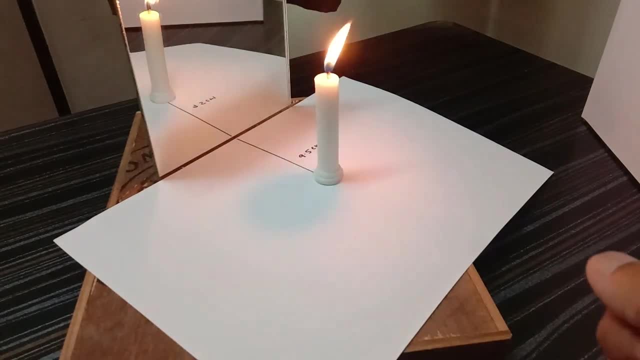 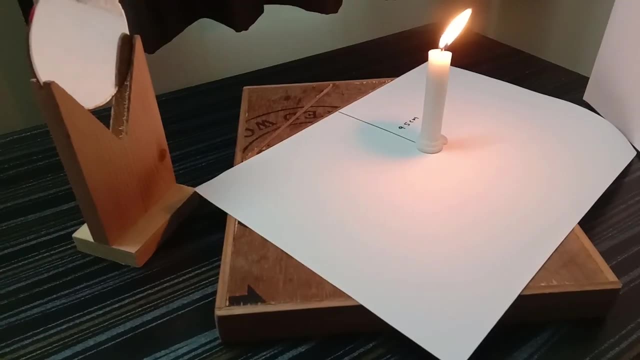 another mirror near it, which is our concave mirror, I would be able to obtain a real image on the screen. So let me show you that. All right, guys. So now what I have done is I have replaced my plane mirror with the convex mirror, which